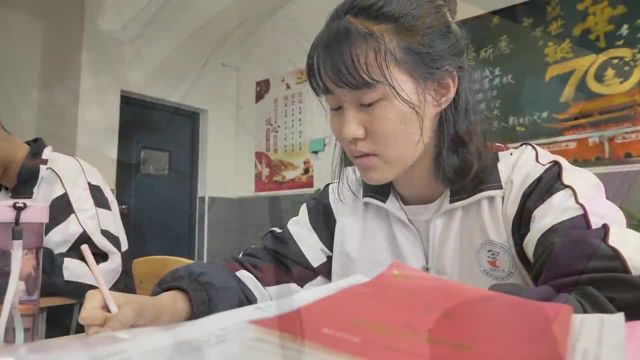 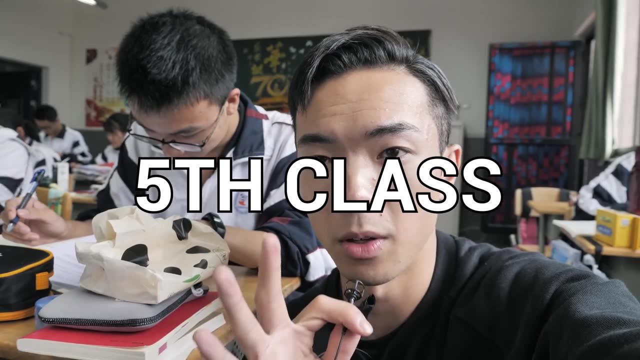 These students are all working towards a common goal, and that's to get a good score on the 高考 so they can get into a good university. Right now it is the fifth period in the morning, so the next one is going to be lunch and it's another self-study period. 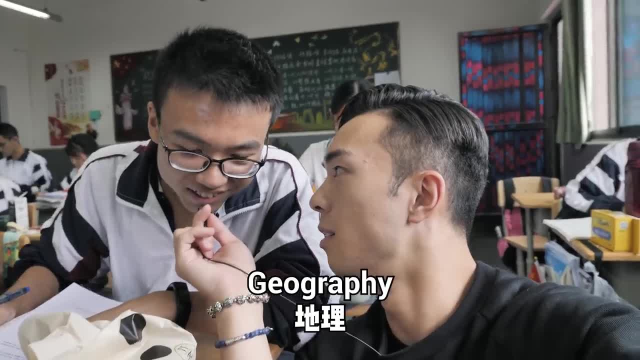 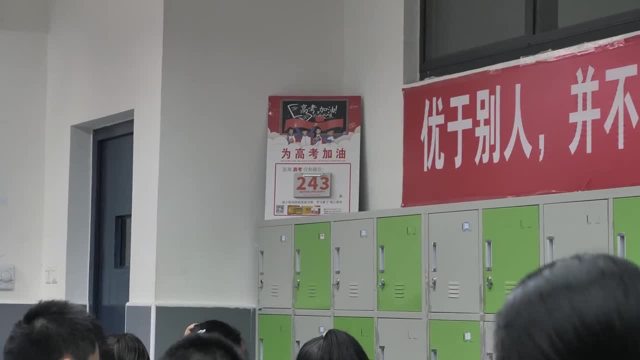 What are you studying right now, 地理? What are you studying right now, 地理? First I'm reading a book and then I'm memorizing the points and then I'm doing my homework. At the front of the class is a 高考 countdown calendar. 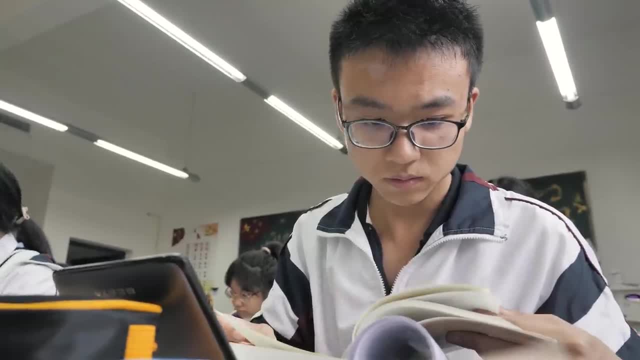 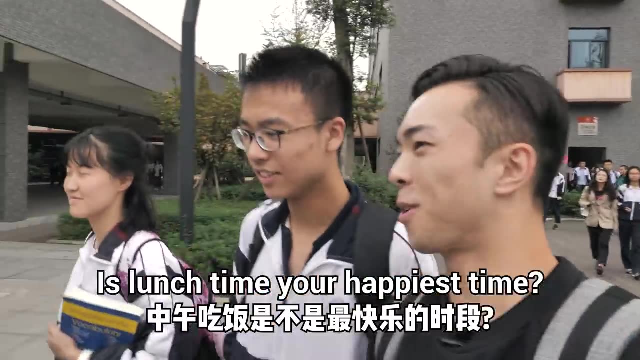 It's a constant reminder to practice perfection. 中午吃饭是不是最快乐的时段? 中午吃饭是不是最快乐的时段? 吃饭还是最快乐的时段. 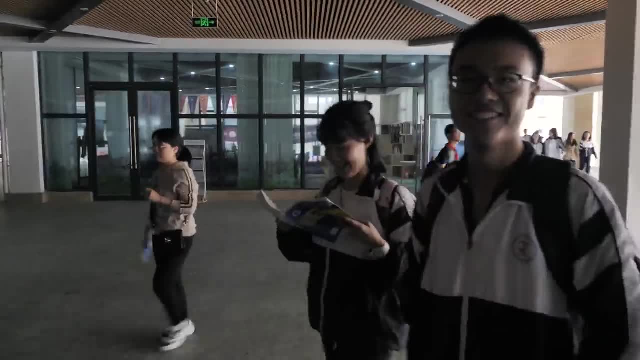 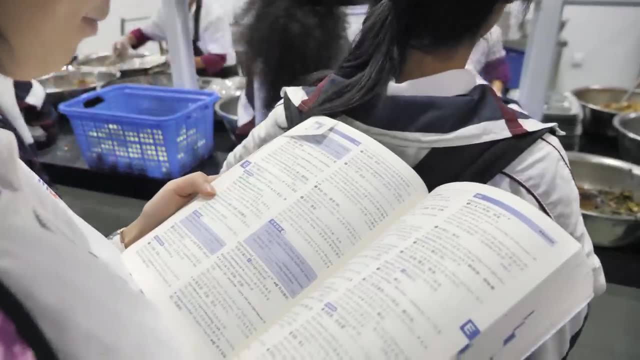 This is a boarding school, meaning the students all live at the school, so food and scheduling is all taken care of by the teachers. All the students have to worry about is getting good grades. All the students have to worry about is getting good grades. 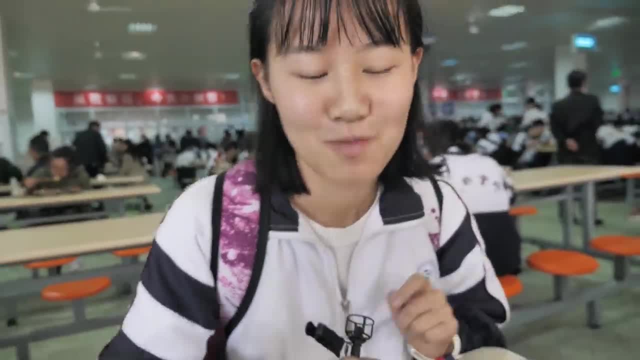 好吃吗? 今天的饭很好吃。. 今天的饭很好吃。 今天好吃。. 你觉得好吃吗? 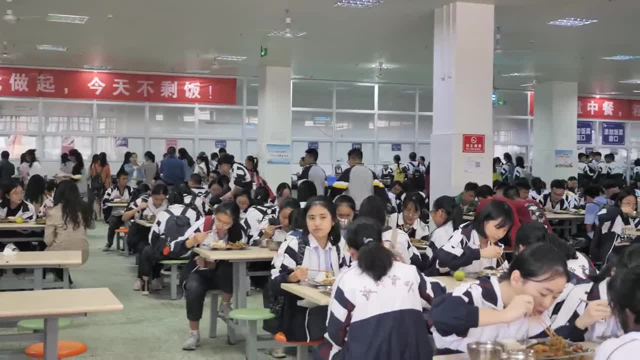 挺好的挺好的。 你可以自己体验一下。 你可以自己体验一下。 算不算最好吃的但还可以觉得压力大吗. 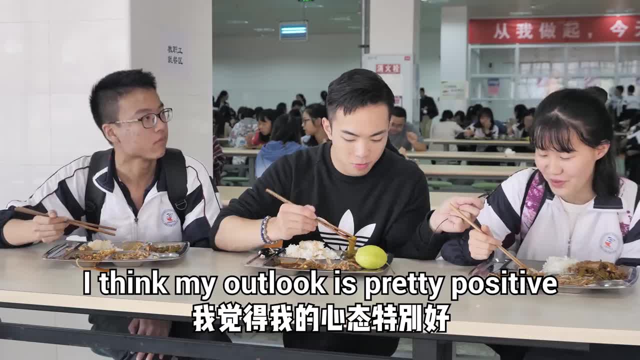 算不算最好吃的但还可以觉得压力大吗? 压力是肯定有的但是我觉得我的心态特别好。. 压力是肯定有的但是我觉得我的心态特别好。. 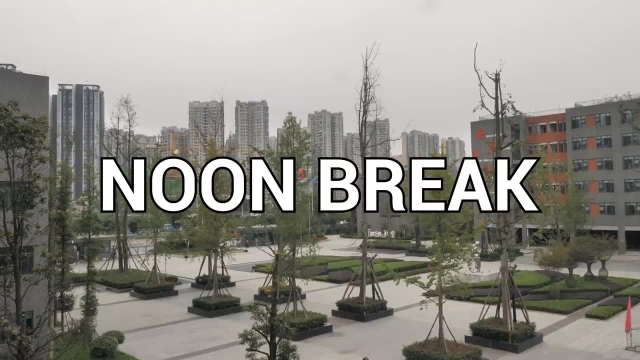 我学的又挺有目标但是又还挺高兴的。. 我学的又挺有目标但是又还挺高兴的。. Right now it's around 1.30.. 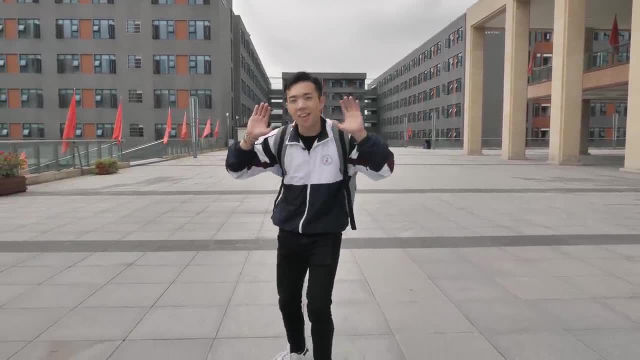 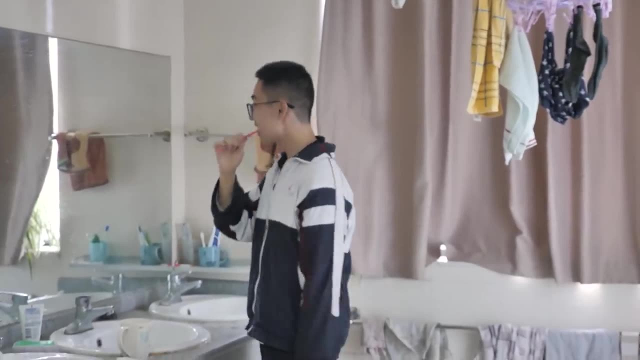 The school is dead silent. It's actually because all the students are taking their afternoon nap for one hour. It's actually because all the students are taking their afternoon nap for one hour. 几个人住啊, 几个人住啊? 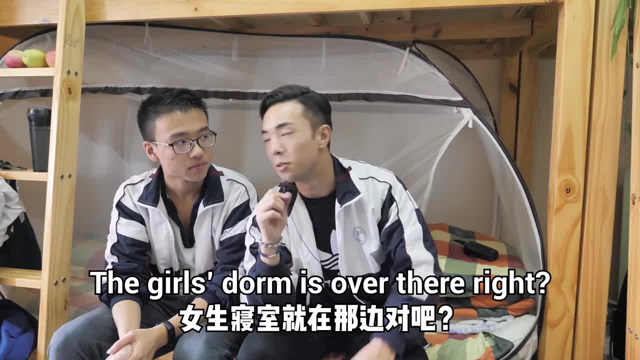 本来是五个的然后有个同学去国外的然后剩下四个。 本来是五个的然后有个同学去国外的然后剩下四个。. 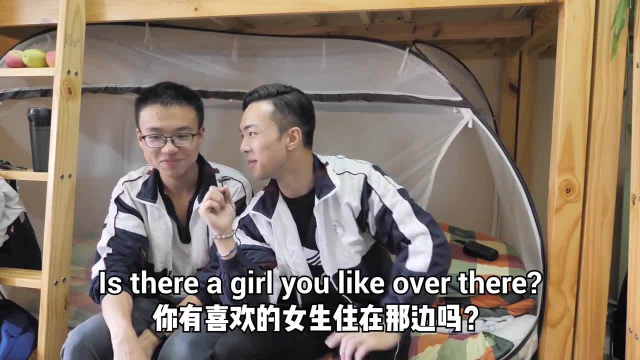 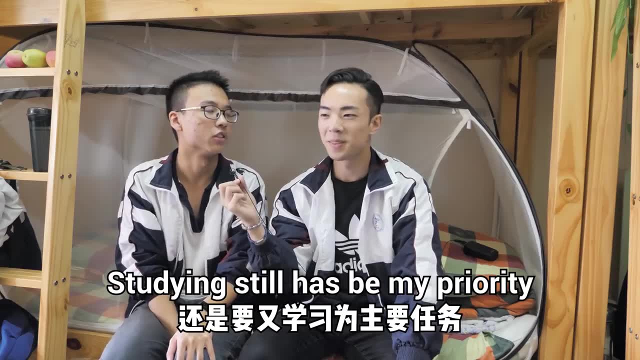 女生寝室就在那边对吧, 对。. 你有喜欢的女生住在那边吗? 没有没有。. 还是要以学习为主要任务。. 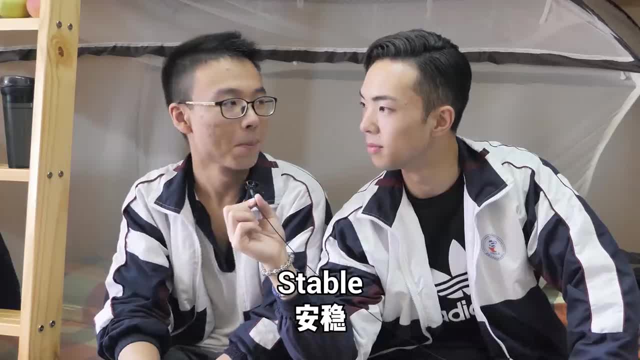 可以用一个词来形容你现在的生活吗? 可以用一个词来形容你现在的生活吗: 安稳。. 跟着学校的安排一起走。. 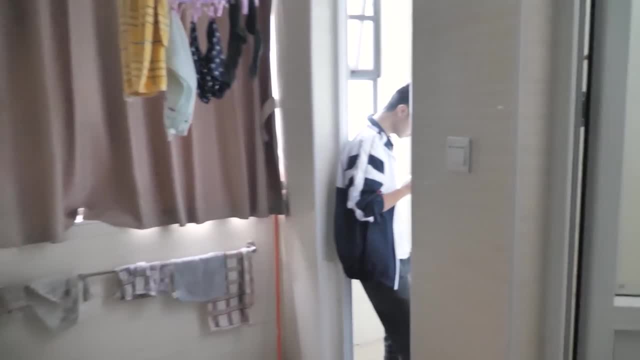 我要脱裤子了。 大家有时间睡觉了。 大家有时间睡觉了。 后面是优秀毕业生班。 后面是优秀毕业生班。. 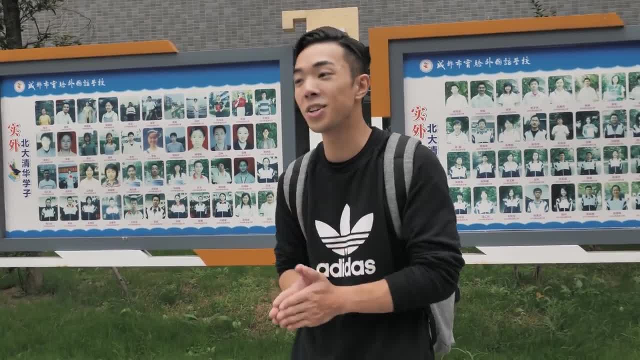 学生在中国最高的学校中。 学生在中国最高的学校中。 中国只有两个学校清华和北大。 中国只有两个学校清华和北大。. 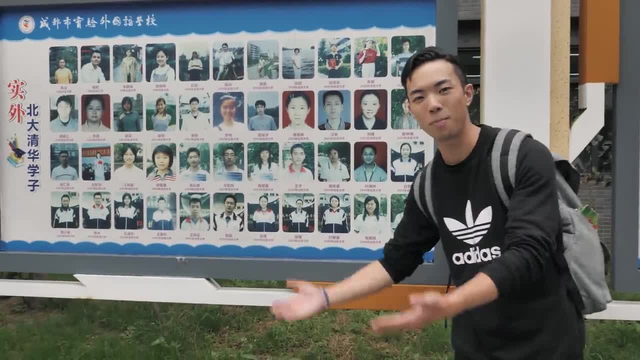 这里是为了激动学生。 每天早上他们可以看着这些学生. 每天早上他们可以看着这些学生 说一天我会去清华北大. 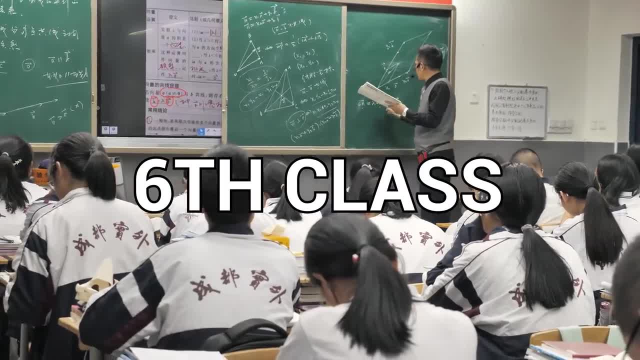 说一天我会去清华北大, 我会努力学习。 现在我们回到课堂了。 现在我们回到课堂了。 我们准备了四堂了。. 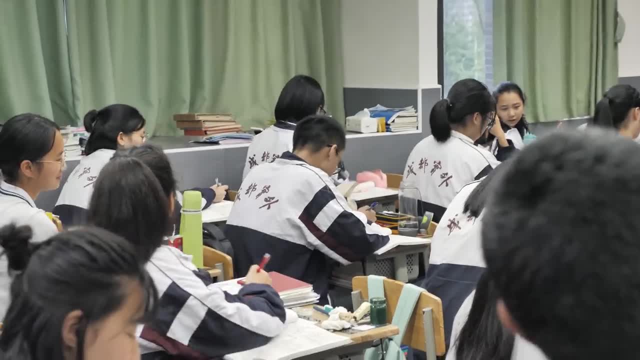 我们预计在下午要吃下午饭。. 我们预计在下午要吃下午饭。. 我们预计在下午要吃下午饭。. 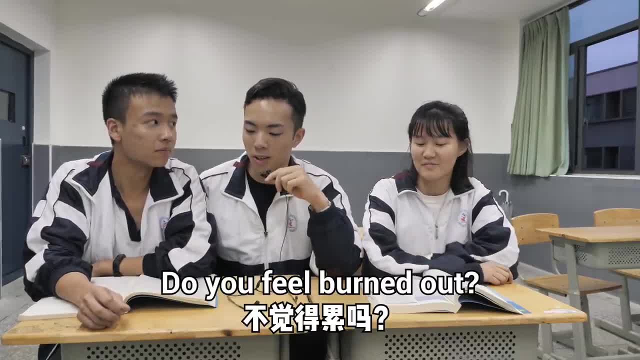 你每天都学这么多东西, 不觉得累吗? 其实不是特别的累, 因为已经深处于其中了。 慢慢地习惯了。. 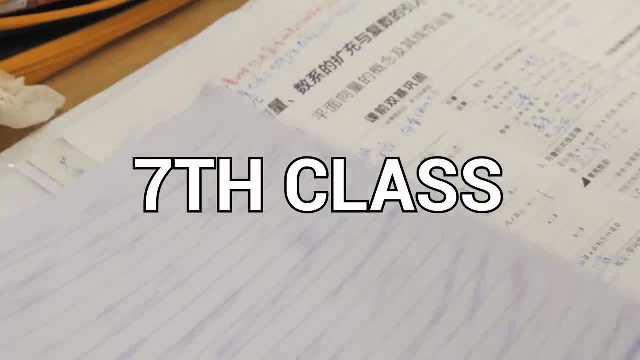 而且学习也是一个收获的过程。 会很愉快的。. 在三天他们都回到了彩排设计院 即使写 MATCH B1。. 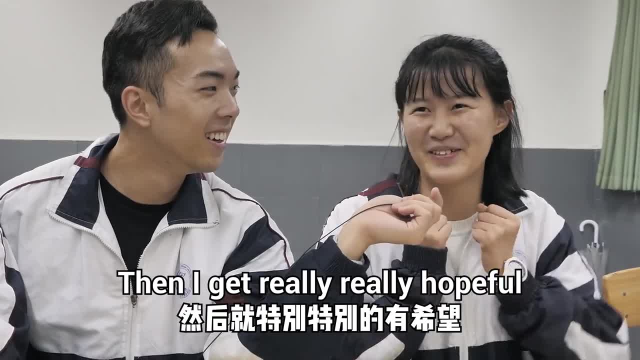 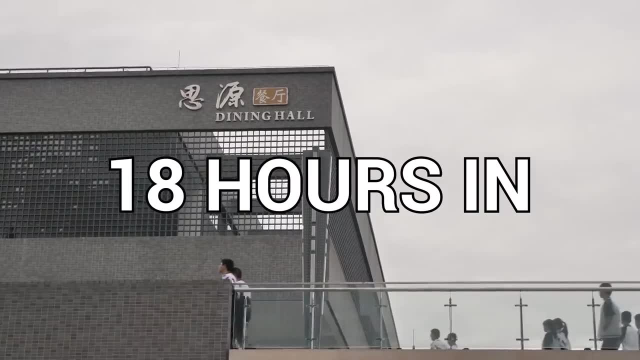 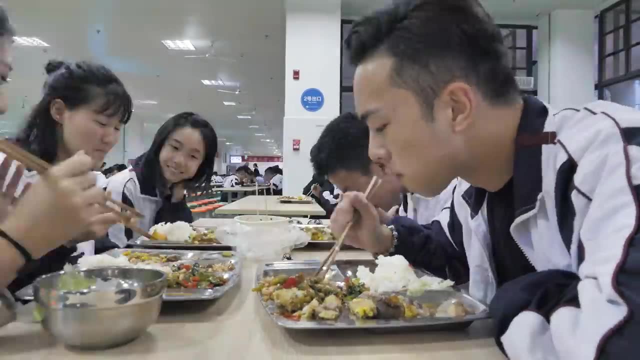 你认为这个是为了续生教权. I want to learn more about my dream and I have a lot of hope for it. Do you know what to eat for dinner? After dinner, students get about 30 minutes of free time. 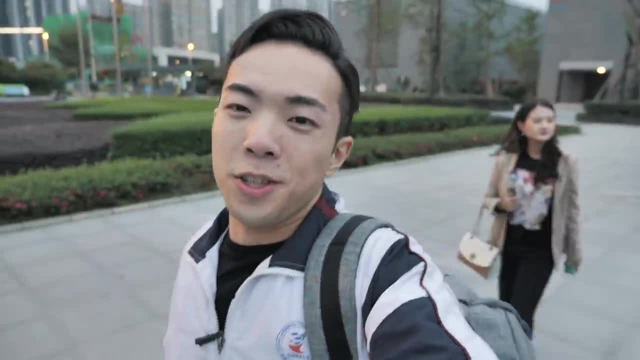 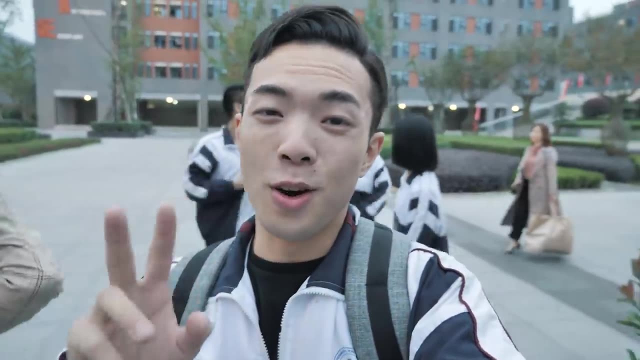 before they have to go back for night class. We just finished dinner. now it's around 6.30.. We're heading back to class for one more night class and two more self-study sessions, And then we'll end around 10.20..